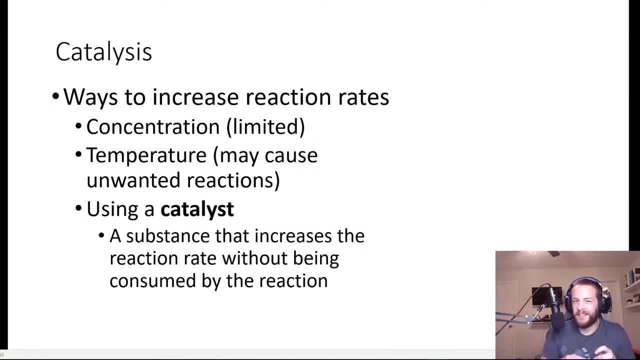 drafted by the Orlando Magic. he was the catalyst that they needed to get to the Eastern Conference finals, right, Something like that. So there's a lot of colloquial usage of the term catalyst, But catalyst has a very, very real and very, very literal definition, And that's what we're going to. 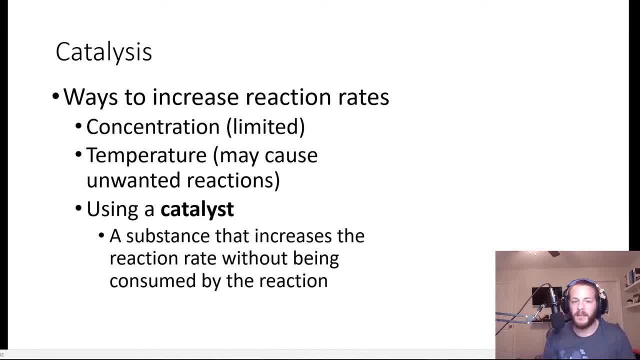 talk about in today's lesson. So a catalyst is a substance that increases the rate of a chemical reaction without being consumed by the reaction, a substance that increases the reaction rate without being consumed by the reaction. So to explain how this works, let's consider: 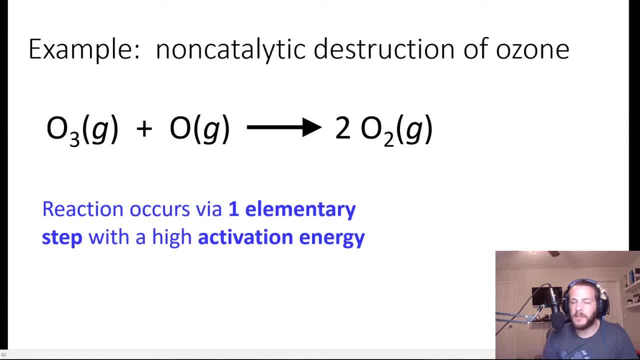 a particular chemical reaction. So the example that we're going to look at in this one is the non catalytic destruction of ozone, whose chemical equation is shown right here. So ozone O3 is a component of the upper atmosphere, right, And it gets destroyed naturally according to this equation, where you have 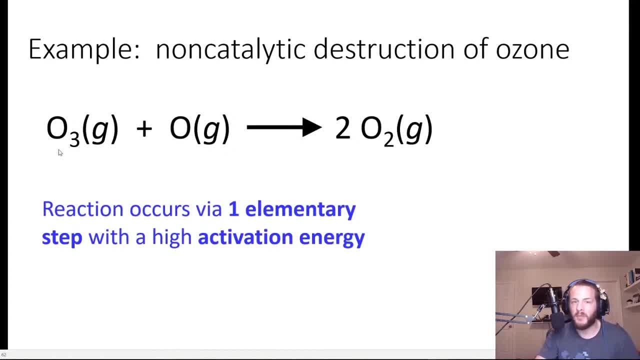 and this is a one step mechanism where you have a molecule of O3 colliding with an individual oxygen atom to produce two O2 molecules. So it occurs via one elementary step And you might think, oh no, the ozone is being destroyed by this reaction. Well, 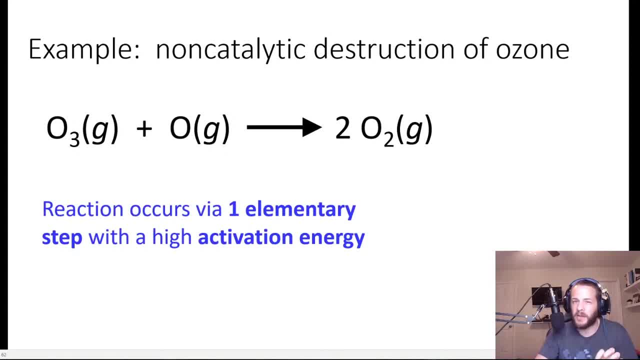 yeah, it is, but it's occurring naturally And this particular reaction is slow because it has a fairly high rate of destruction. So it's a very, very natural reaction And it's a very, very high activation energy. Right Now, imagine that there's a catalyst introduced to this reaction. 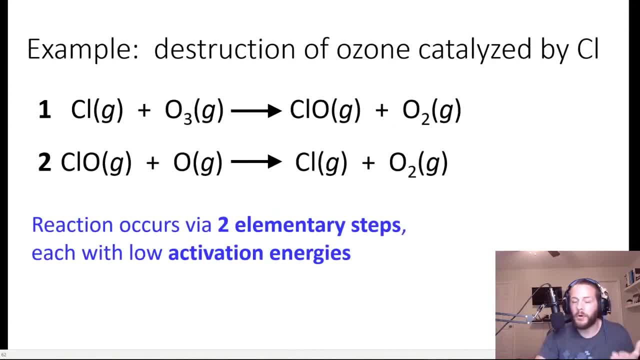 which happens a lot because of manmade chlorofluorocarbons, which I'm not trying to go on some environmental rant or anything like that, But this is just an example of of one reaction that's catalyzed by by manmade chlorofluorocarbons, So the destruction of ozone can actually be. 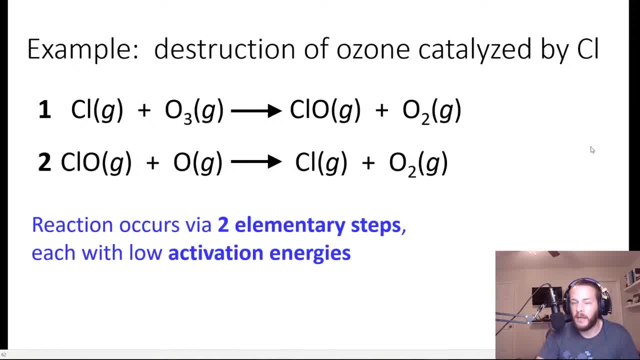 sped up and catalyzed by chloro And the chlorine atoms. again, they come from fluorocarbons. So the way that chlorine-catalyzed destruction of ozone works is by a two-step process. right In the first step you have a chlorine atom colliding with an ozone molecule to produce 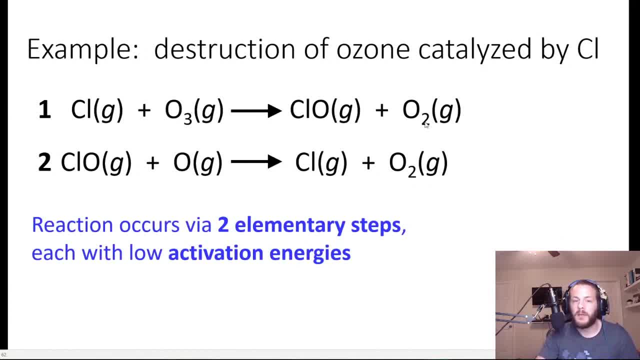 CLO and an O2 molecule, And then, in the second step, you have the CLO molecule that was produced by the first step, colliding with an oxygen atom to yield one chlorine atom and one oxygen atom. So notice that the initial definition of catalyst was something that increases the rate of a. 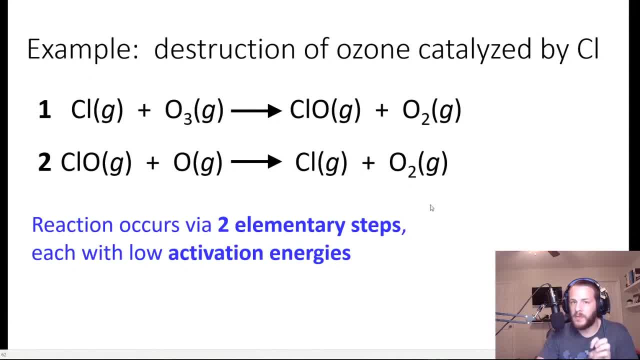 chemical reaction without being consumed, right? So in this case, the chlorine, that's the catalyst. right Now, notice that the chlorine is introduced as a reactant in the first step and it's a product of the second step, right? 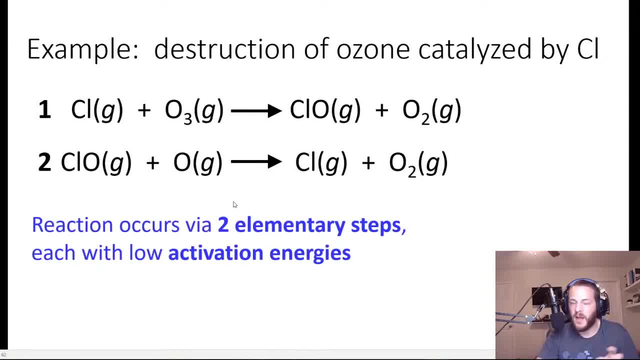 So it's regenerating By this mechanism. So it's not actually consumed. It's consumed for a very short period of time in that first step, but it's reproduced in the second step. So this mechanism, this chlorine-catalyzed destruction of ozone, occurs via two elementary 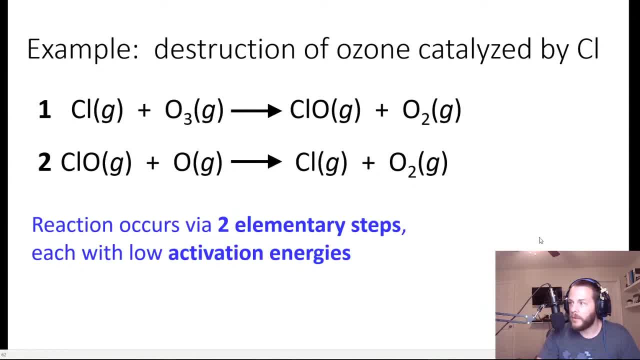 steps rather than one, And each of those two steps have low activation energies. Now you might be thinking: how does adding a second step to a mechanism going to speed up a reaction? It's kind of counterintuitive. You would think adding a second step would actually slow things down. but that's actually. 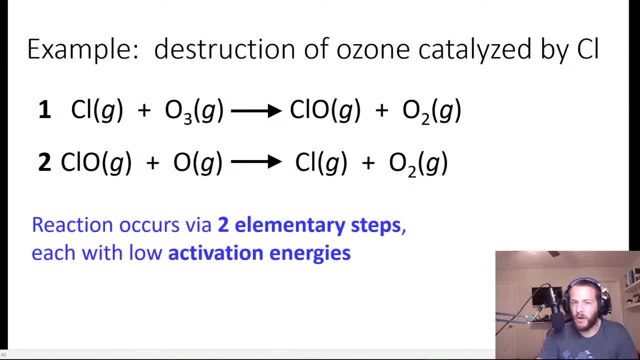 not the case because, remember, it's not about how many steps there are, It's about how fast your slowest step is, how fast your rate-limiting step is, And so if we look at this, just to show you, for instance, if we cancel out the catalyst, 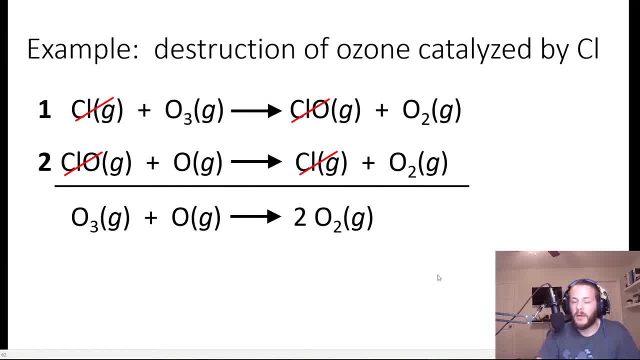 and we cancel out the CLO intermediate. notice that if we add these two reactions or these two elementary steps together, we do indeed get the same rate of reaction. We do indeed get the same reaction that we had before. right, The one that occurred in one step, where you have O3 plus O yields 202, right. 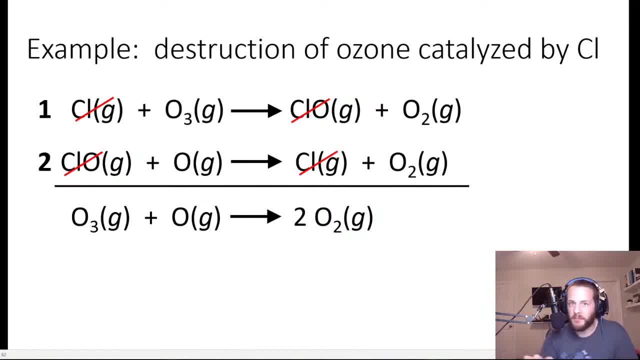 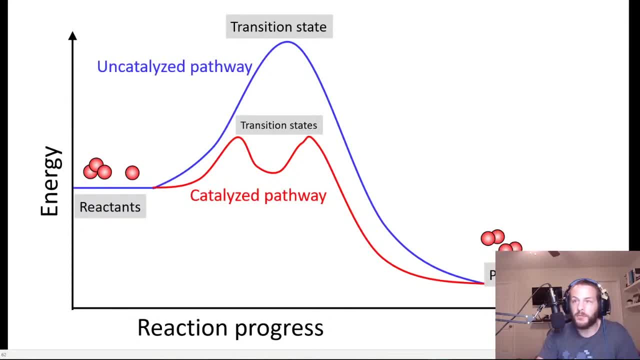 So I just wanted to make sure I put that in there, that they're both the same reaction. They're just occurring by two different mechanisms, right, And so if we look at a diagram of this, this is another one of those energy versus reaction. 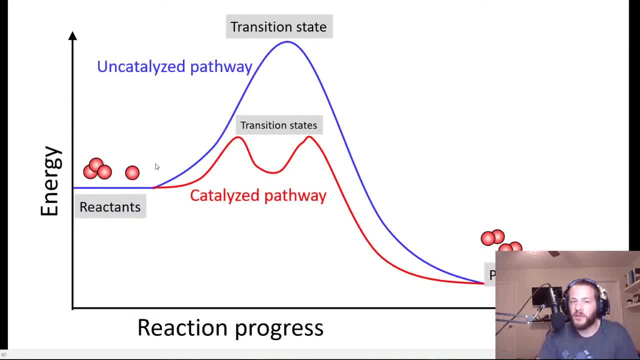 progress diagrams. So the graph shown in blue here, this represents the uncatalyzed pathway, the single step mechanism. The single step mechanism that occurs naturally right And it has a high activation energy, because this little hump right here is really really. 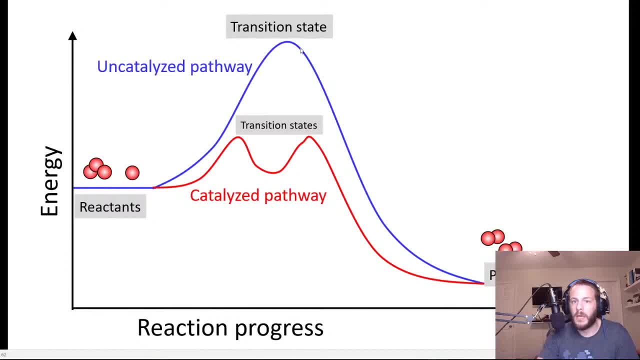 high up right And notice that there's one of them. There's one of those peaks right here, right, Which makes sense because there's one step right And in red. this represents the catalyzed pathway, where we have two steps right. 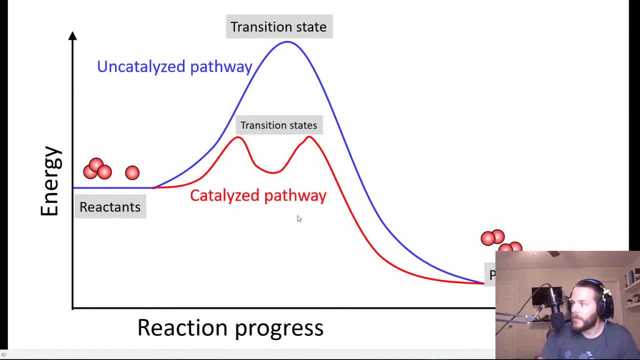 Two humps, two local maxima right. So notice that we have, like I said, these two different Pathways here: the uncatalyzed pathway, that has a very high activation energy for its rate limiting step, which is the only step, and the catalyzed pathway which, even though, 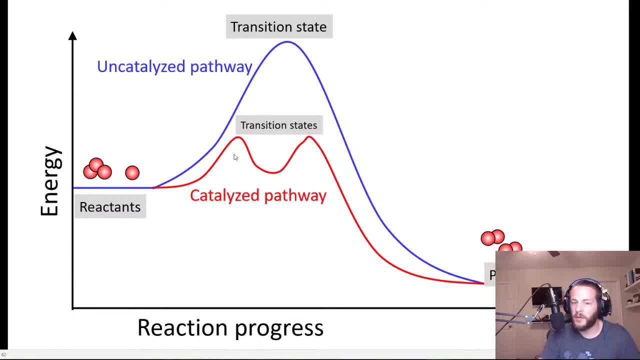 it occurs via two steps. each of those two steps has a very low activation barrier, And so, therefore, the catalyzed pathway is going to be the faster reaction. So, in this case, the reaction that is being catalyzed is an unfavorable one. 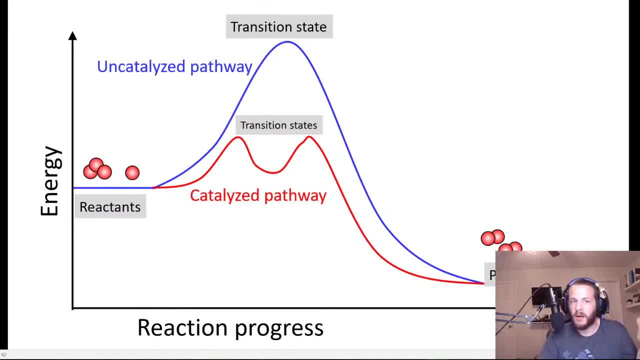 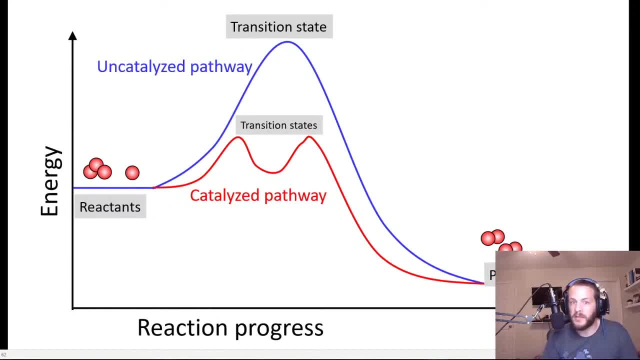 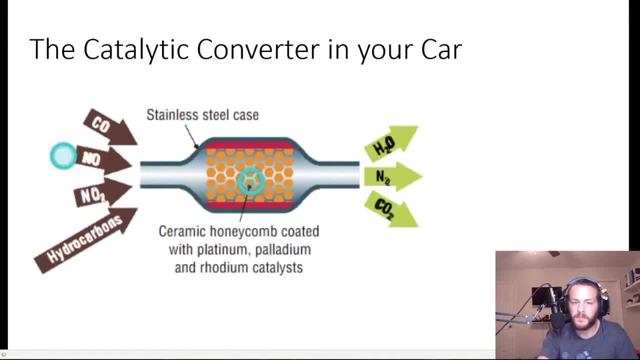 But other times, oftentimes, we actually intentionally use catalysts to speed up reactions that we do want to occur. We speed up reactions that we do want to go faster. So, for instance, one of those such reactions is the catalytic converter in your automobile. 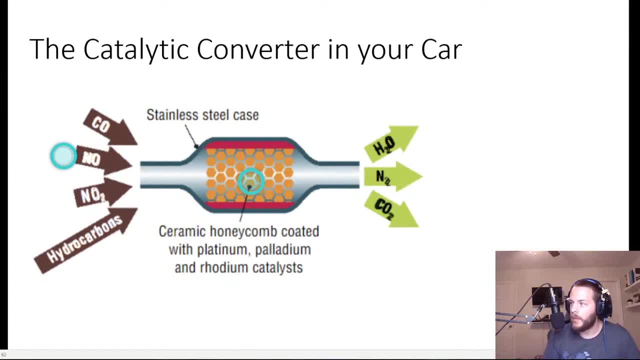 So you've probably heard the term catalytic converter before, but you may or may not have given much thought to it. You may not have given much thought to what that term actually means or how it works. So the catalytic converter is a component of your vehicle that's connected to your exhaust. 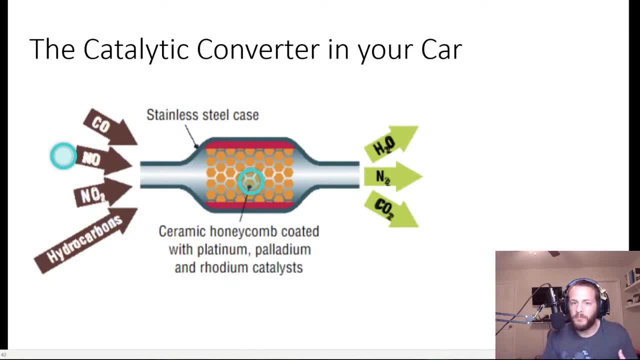 Right. So your engine. it burns up some fuel and then the fuel turns into exhaust and that exits your vehicle. Right Now, in the engine of a car there's combustion of the fuel, but the combustion is generally not complete. 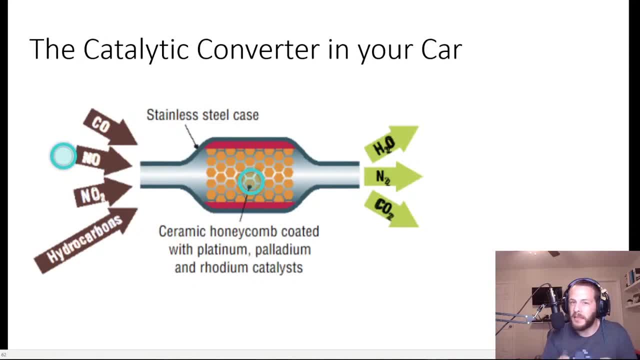 There are plenty of incomplete combustion products. It's not a completely efficient process, Right? And so there's a couple of things that come out of the car that are really nasty, like carbon monoxide, like nitric oxide, like nitrogen dioxide, fragments of the fuel that just didn't 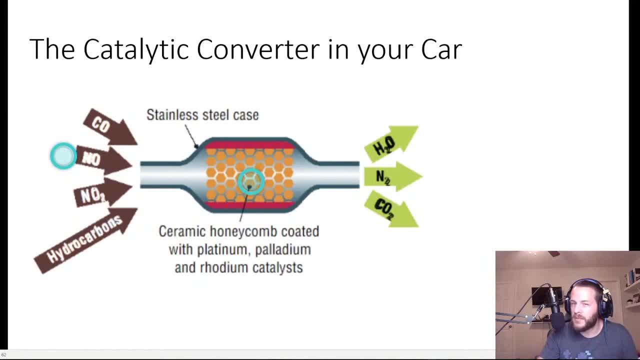 get burned, all those kind of things that, if they were released into the atmosphere, well, they're not so good, Right. They're not so good for the environment, Right. And so the way that the catalytic converter works is it has this catalyst. 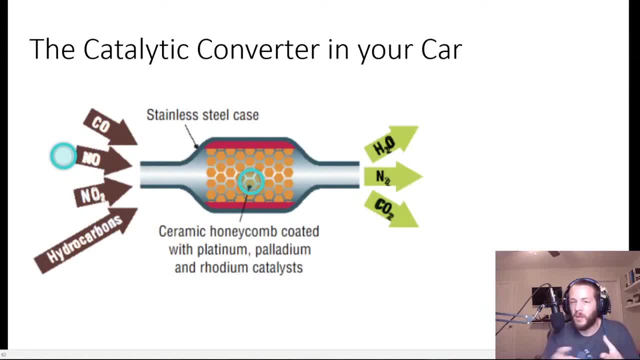 This high surface area ceramic structure and within that high surface area ceramic structure- let's try saying that 10 times fast. you have these metal catalysts. You have platinum, palladium, rhodium, little bits of that metal, Right? 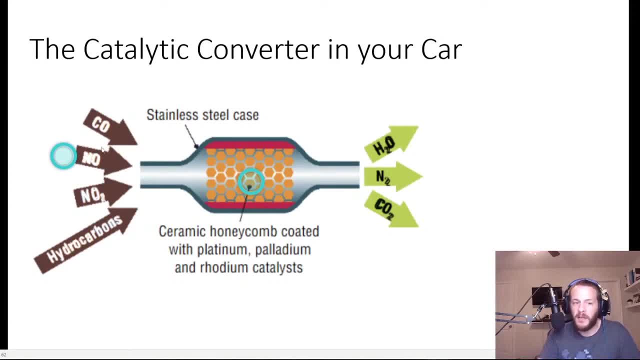 And that metal catalyzes the reaction of these nasty materials that we don't want into the atmosphere to make things like water, which is harmless, Right, I mean we drink it. It makes up over half of our bodies by mass Right. 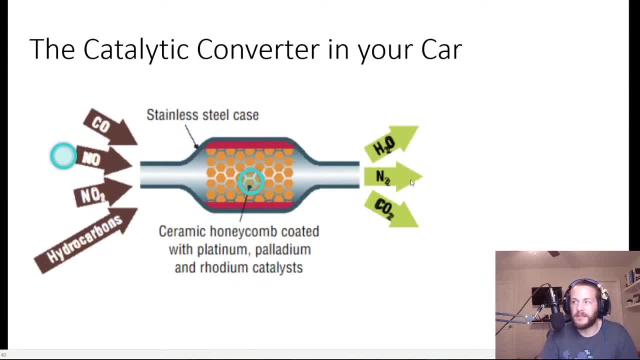 Nitrogen gas. Nitrogen gas is very inert. It's pretty much harmless. It makes up 78% of the air that we breathe, So nitrogen is infinitely preferable than something like nitric oxide or nitrogen dioxide, which are both toxic And CO2.. 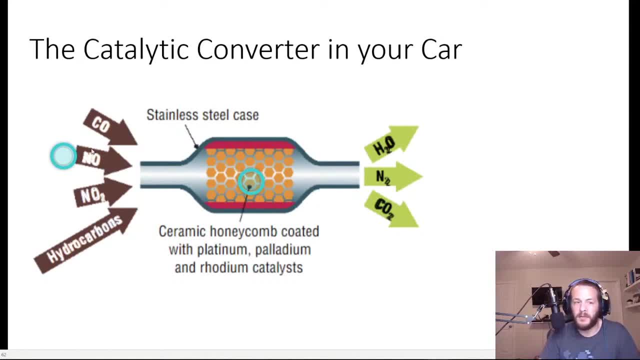 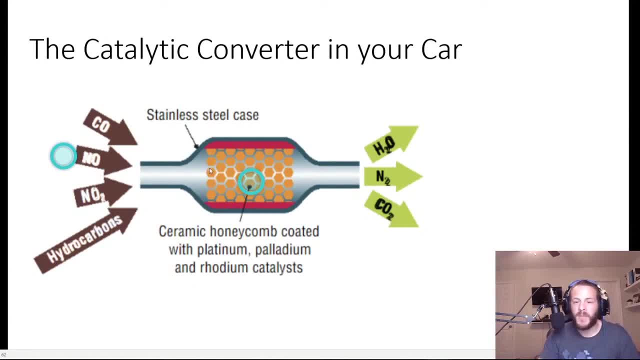 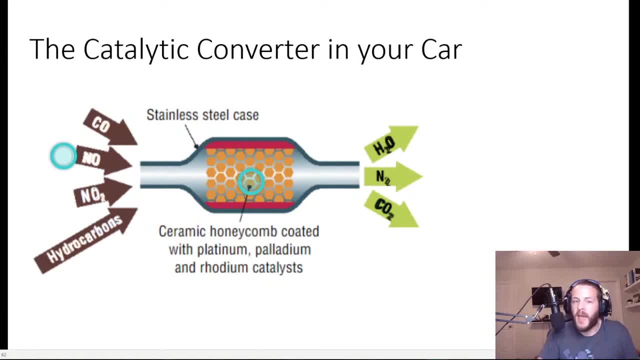 CO2, carbon dioxide, much better to have in your atmosphere than carbon monoxide. So the catalytic converter uh takes advantage of catalysis uh to convert certain materials that may be a bad idea uh in the atmosphere. 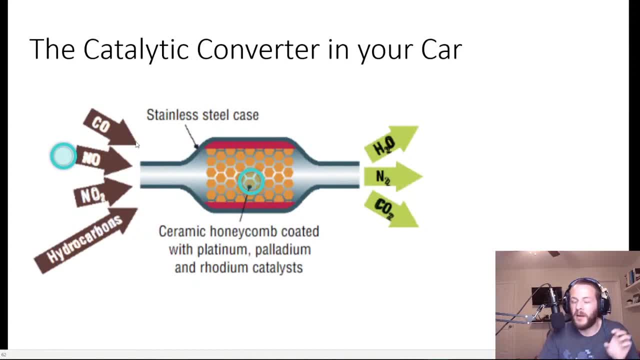 So, like I said, co2, not really toxic, But if youSo, we have seen CO2 onions before. It's aFeExpicaIty: things happen. convert things that are bad to things that are either good or not as bad. so that's how your. 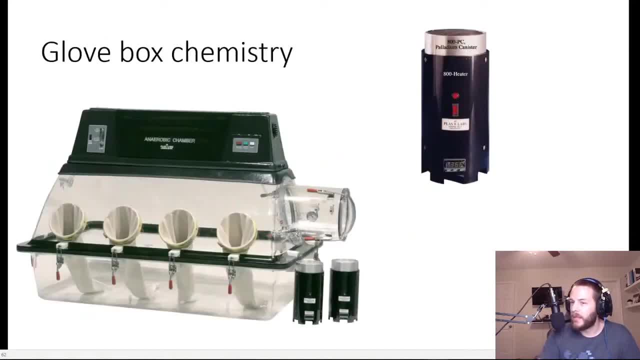 catalytic converter works and there's another uh sort of thing with catalysis that i wanted to tell you guys about now. this is from from personal experience. so at my last job- not the job where i'm working now, but, uh, my last job- i did a lot of work with um, inert atmosphere, chemistry, like a lot. 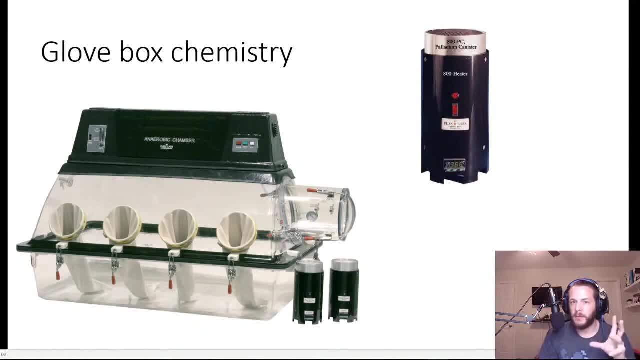 of. i worked with a lot of air sensitive and moisture sensitive materials like things that if you, you know, open the container in the presence of air it would ignite or it would ruin the material. so pretty dangerous stuff and one efficient way to handle these kinds of things. 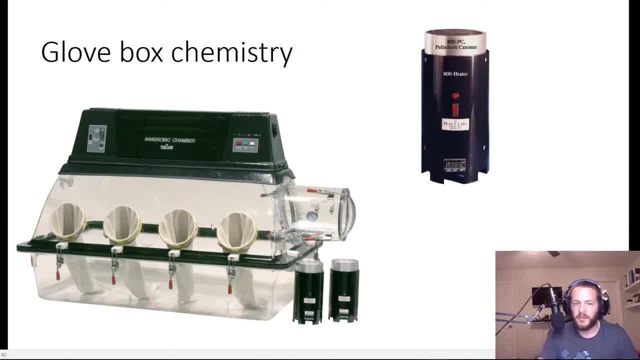 is by using a glove box or an anaerobic chamber, and this is actually the kind right here that i used to use every single day and, as you can imagine, it can be pretty, pretty difficult to reach with those gloves and and try to do delicate work that way. 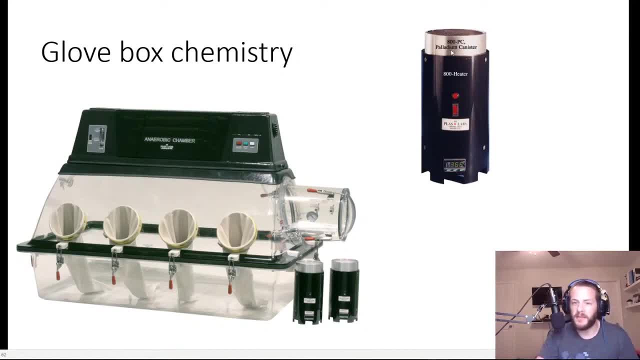 but one of the things that i wanted to bring to your attention is this thing right here, this thing, it's it's called the heater, or the. the blower is as it's often called, so the way that this works right. so obviously you have this chamber and you want to keep the oxygen out of it. 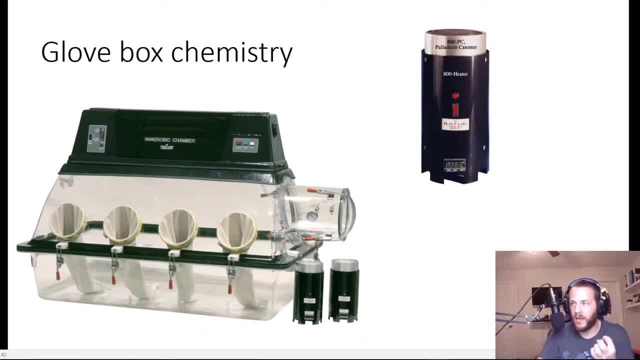 right, because oxygen is the component of the air that reacts with air sensitive materials. right? so you have this, this unit, here, and what what it does is it takes the atmosphere that's inside the glove box and it sucks it through the bottom and it pushes it up through the top. 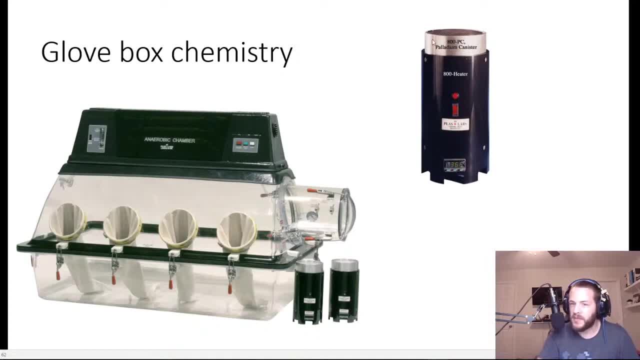 right and at the top, notice that there's this metal thing. this is a palladium canister. so it's this metal canister that has a bunch of little palladium pellets in it, right, and what that does is it catalyzes the reaction of hydrogen with oxygen to produce water. so whenever you are 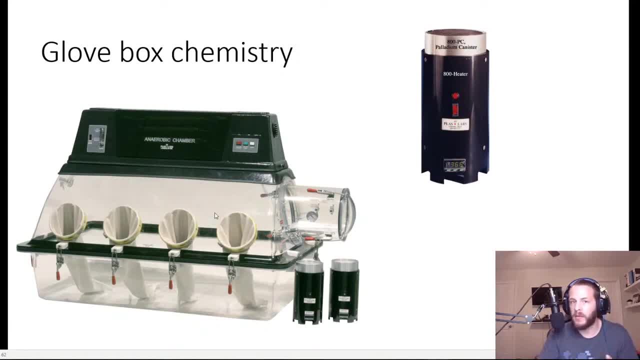 filling this chamber with gas. the gas that you fill it with is, uh, part part of it. most of it is argon, but the rest of it is hydrogen. so you intentionally introduce hydrogen gas in here to react with any oxygen that leaks in, just incidentally, because no matter how hard you 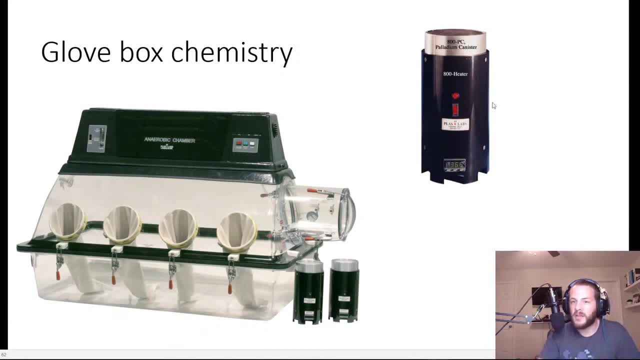 try, there's definitely going to be some oxygen that leaks in, so that oxygen reacts with the hydrogen that you already have in there and it's catalyzed by this palladium canister in here and it produces water. now, it's also not good to have water in your glove box either. 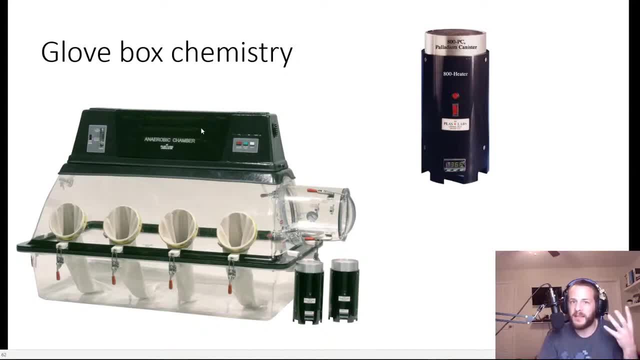 but that's why there's this thing up here. this is called a drying train. it's basically like these canisters: you push a button and it cycles the atmosphere through the drying train and it's packed with molecular sieves that trap the water. so it's pretty cool stuff. it's pretty. 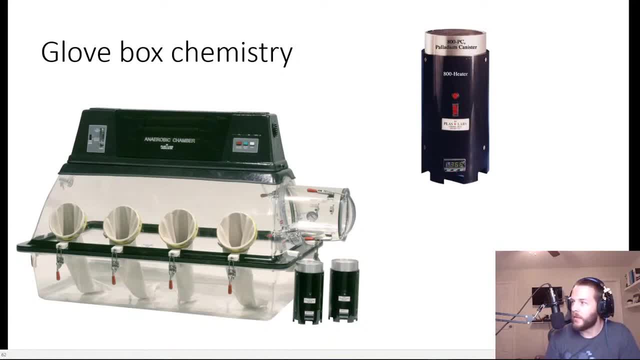 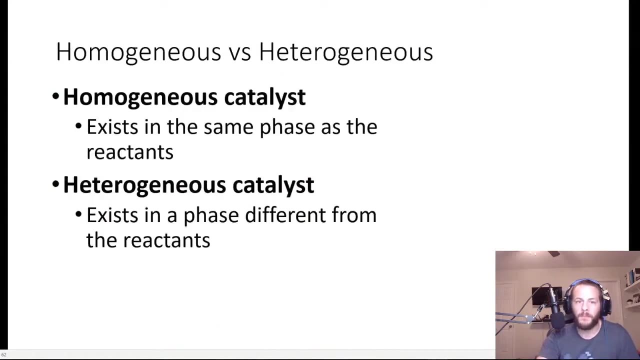 cool stuff. it's a very um elegant solution to the problem of air and moisture contamination within a an inert atmosphere anaerobic glove box. so just another example of catalysis- uh doing work for us. um now, one thing i wanted to touch on is uh, two different. 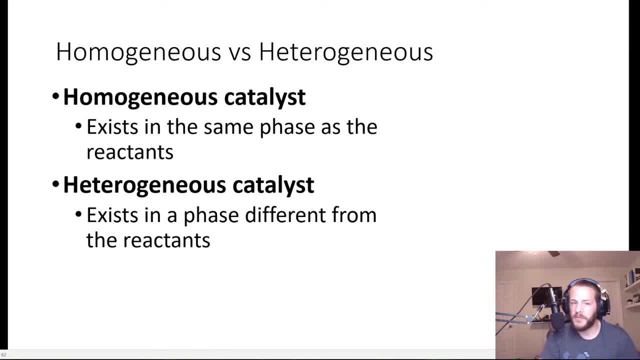 types of catalysis, uh, which are homogeneous and heterogeneous. so, uh, and these are pretty straightforward: a homogeneous catalyst is a catalyst that exists in the same phase as the reactants, and then, on the flip side, you have heterogeneous catalysts, which exist in a phase that is different from the reactants, right? so an example of homogeneous catalyst that would be like: 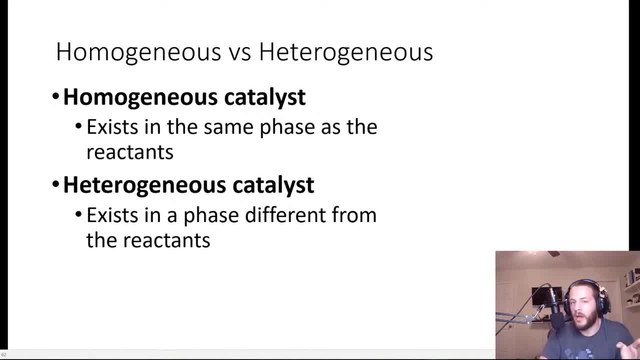 the chlorine that gets introduced into the atmosphere. that catalyzes the destruction of ozone. because the chlorine is a gas, the ozone is also a gas. they're the same phase, right. heterogeneous catalyst. that would be like the solid bits of metal that are suspended in that ceramic structure. 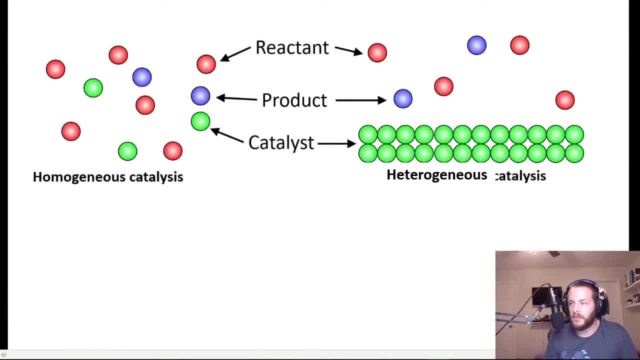 in the catalytic converter of your automobile. so just as a little diagram here, we can see these two different types of catalysts here. homogeneous catalyst, as i said before, is the the same phase as your reactant particles. in this case they're both gases and then in the 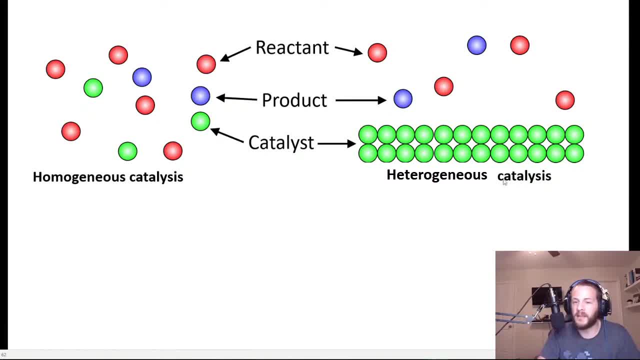 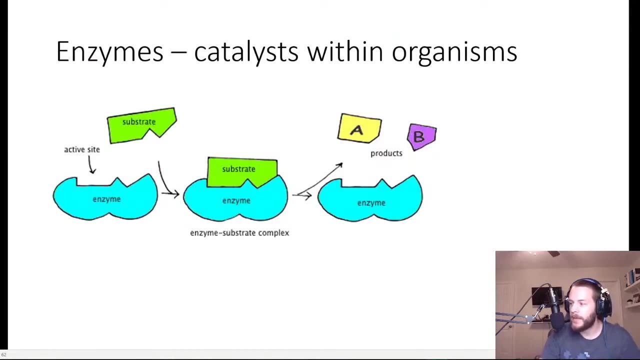 uh, a heterogeneous catalyst. um, in this case we have like a solid catalyst, like with the palladium or rhodium or whatever catalytic converter: different phase of matter as your reactant particles. so the last thing that i wanted to talk about, just as i suspected, the stream is: 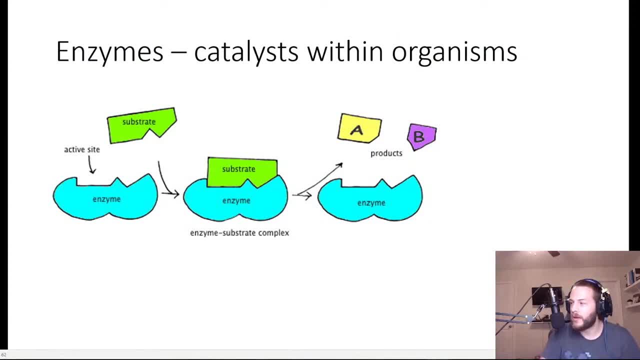 going pretty quickly. so our enzymes, which are catalysts within organisms. so if you think about all the tools that chemists have available in the lab to speed up chemical reactions, like increasing temperatures really high, increasing pressures, you know, increasing concentration, things like that, a lot of these- 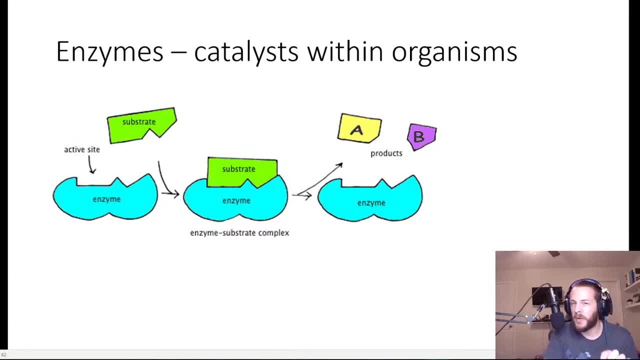 techniques that we use in the laboratory are not available to biological organisms because, you know, high temperatures and high pressures and stuff like that would damage living cells. so we don't we, they don't have those organisms, don't have those methods available. but what they do have are these things called enzymes. you've probably heard the term enzymes before.